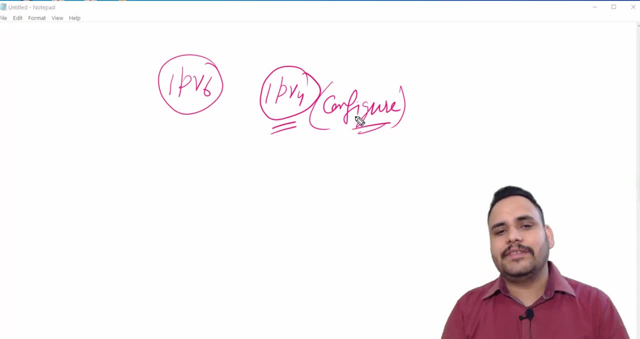 and how to do configuration on routers and PCs. So our today's topic is IPv6, Internet Protocol Version 6.. First of all, why we need IPv6? Actually, in our IPv4 addresses, if we talk about IPv4, then in IPv4 address we have a. 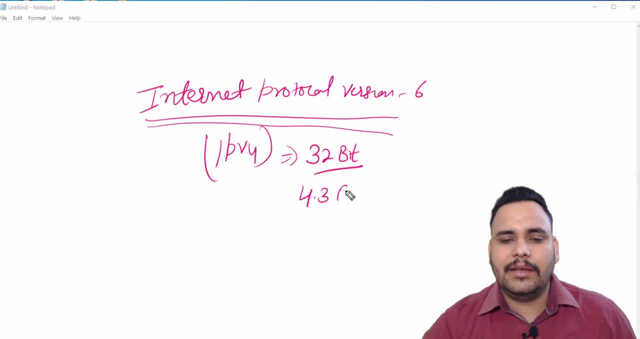 We have a 32-bit address and 4.3 billion IPv4 addresses are there And we know that all over the world population is going to be 8 billion. Within just years or two years, it will become 8 billion. And we are using private IP address, we are using subnetting. 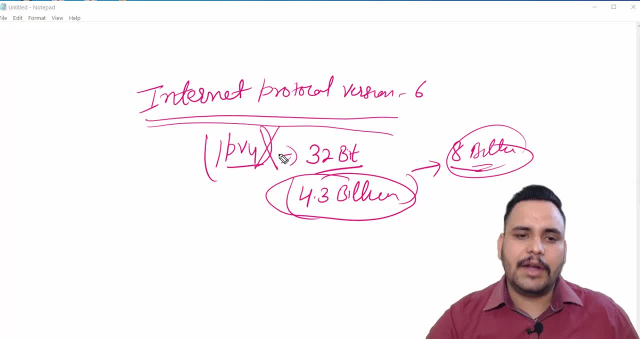 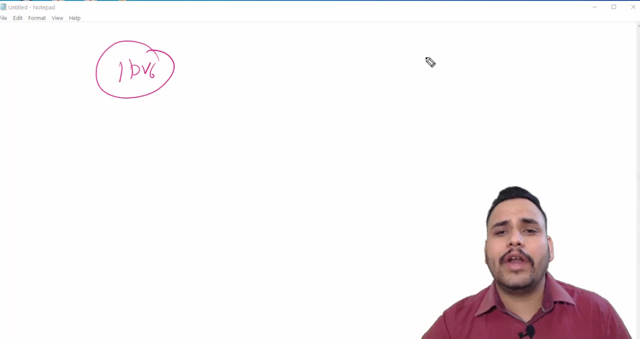 But at one time IPv4 address are going to not be used in the market because it is already used, So why we need one new IP address? That name is IPv6.. So what is the difference between IPv4 and IPv6? In IPv4 it was 32-bit address, It was the decimal address. It was represented. 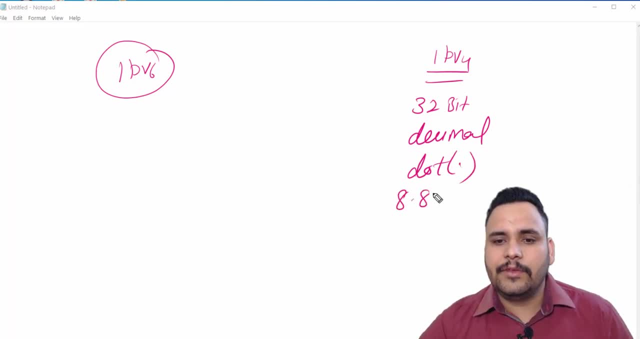 by dot. It was represented with 4 octet. It has classes and we have done with classes subnetmask And in IPv4 address is what we have learned about Classes is done. dot 4.3 billion, IPv4 address approximate. So in IPv6 it is 128-bit address. It is in the hexadecimal format. 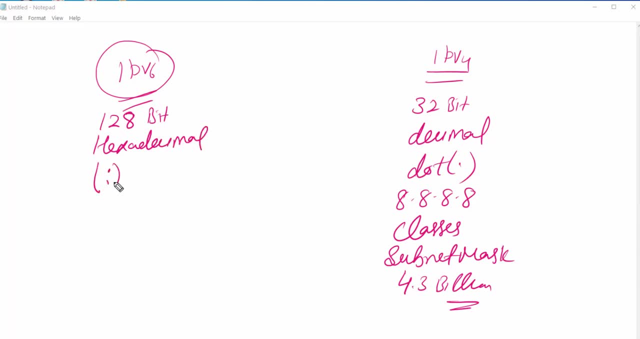 Okay, It is represented by colon. It is represented like this: 16 colon, 16, 16.. So it is a huge and large IP address. It has no concept of classes. Okay, Instead of subnetmask, IPv6 is using CIDR value, Like we call it, prefix length, Like in IPv4 we were using. 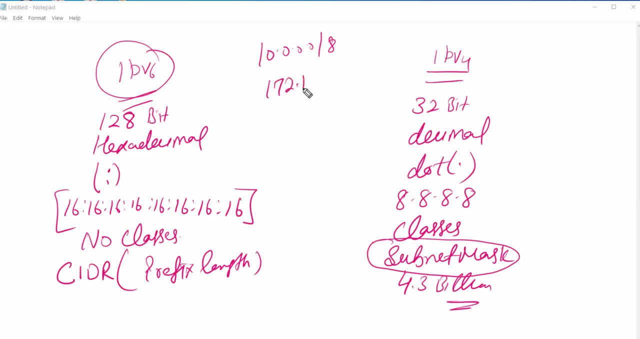 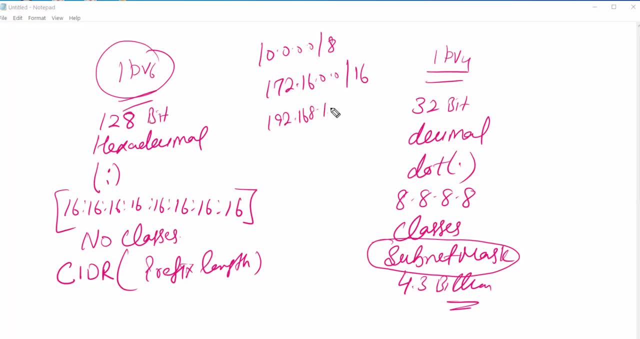 172 16 0 0 slash 16.. 172 16 0 0 slash 16.. 181 172, 169, 169.. 182 169, 169, 168.. 181 169, 168.. 181 0 0 slash 24.. 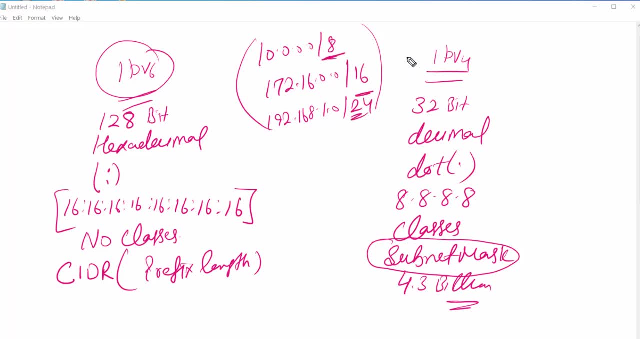 181 0 0, slash 24.. diagonals, And after that we will convert this value into subnetmask like sounded like: 2 5 5 0, 0, 0, 1, 1 and 2 5 5 0, 2, 5, 5, 0 and 3 times 255. 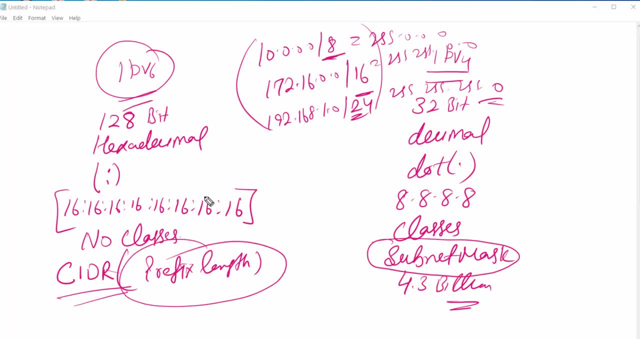 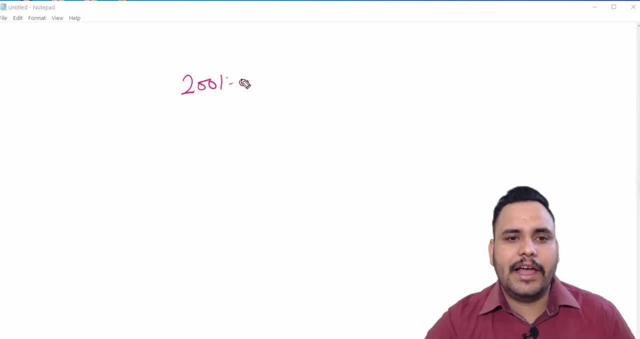 But in this IPv6 we can only choose prefix length. Okay, So how to write IPv6 address? Okay So, first up all to example. This is my IPv6 address. I am using IPv6 address 00000001 and 1,2,3,4,5,6,7,8. ok, so 8 hexes are there, so in this I can choose. 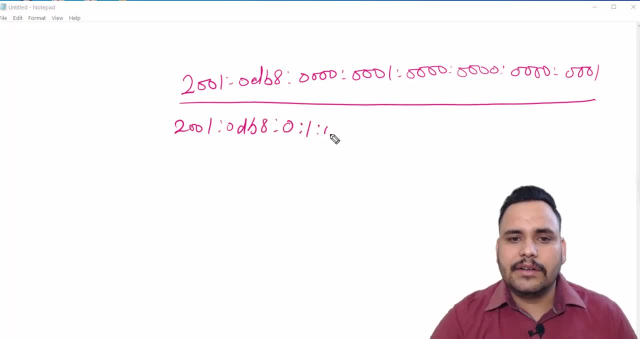 like 0db8 0- 1, 0, 0, 0, 1. like instead of 4: 0, I can put single 0, ok. so if you want to shortens the expression of IPv6 address, you can also use like this: 2001 0db8 0- 1 double colon. 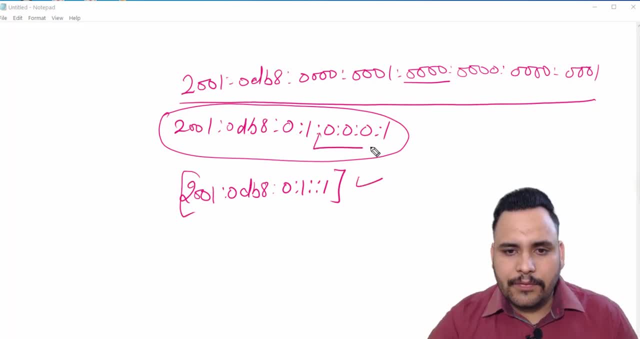 1, like group of 0, can be represented like this, represented with double colon. but, for example, sometime we got 2001 001, 0.0012345671, so now we have two group of zeros. ok, so you can write this IPv6 address like this: or you can write 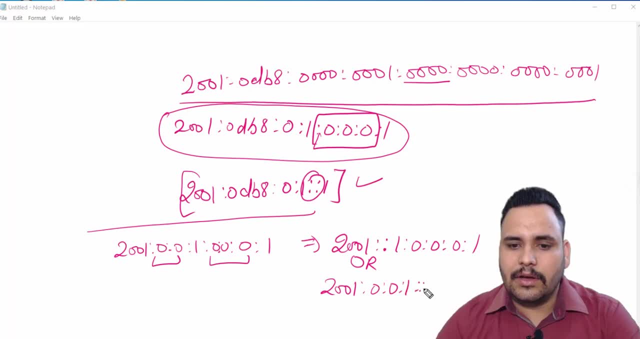 this 00000001, but you are not allowed to use two double columns like 2001 001, 001. this is wrong because then router will confuse like which part has two zeros, which part has three zeros. so this is the expression for shortening the router. now, for example, I was writing IPv4.